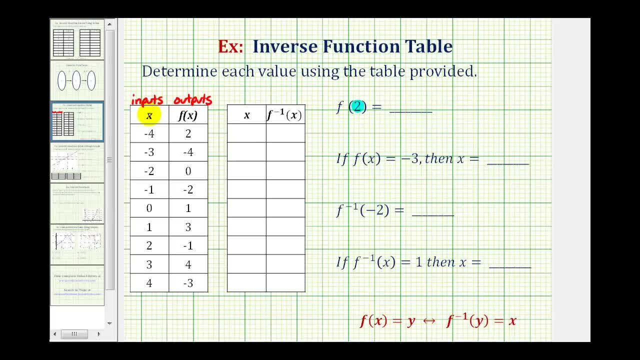 or the x value for function f. So if we go to the table and look for the input of 2 or the x value of 2, notice how the output is negative 1.. Therefore, f of 2 is equal to negative 1.. 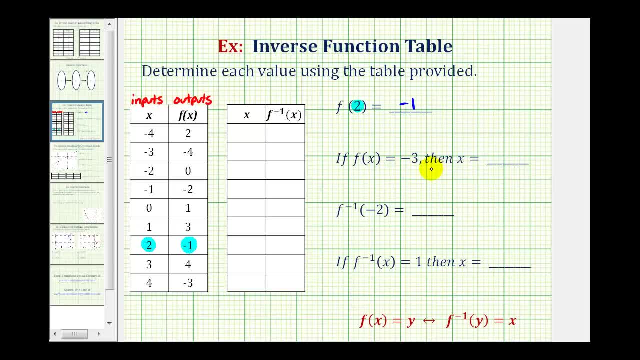 Next we're told that if f of x equals negative 3, then determine the value of x. So now this negative 3 is the output of the function f. So, going back to the table, we're looking for negative 3 in this column here. 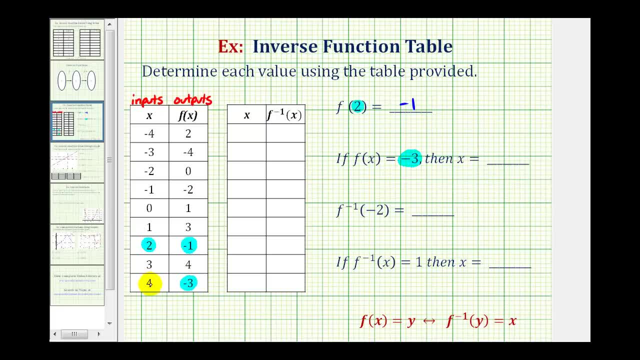 Here, it is Notice, when the output is negative 3, the input or x value must be 4.. So x equals 4.. Now, these last two involve f, inverse of x. So even though we're not required to, let's go ahead and complete this table. 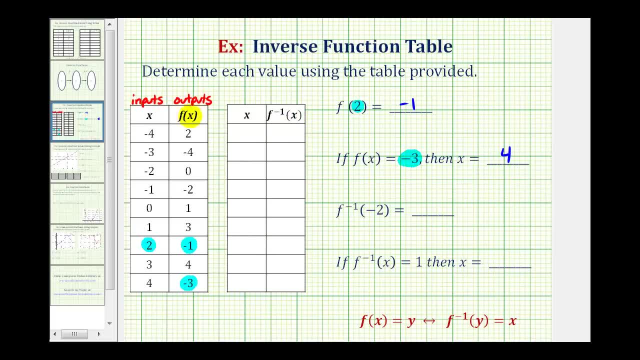 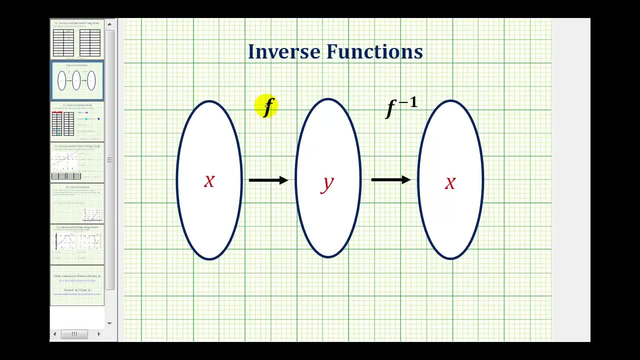 of values for the inverse function. Remember, the function f of x and f inverse of x undo each other, which means if x is the input into function f and y is the output, these y values become the input into the inverse function, which return the original value of x. So, going back to our tables, these will be the inputs. 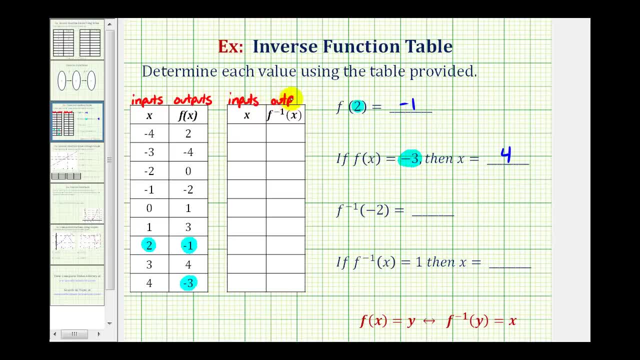 into the inverse function, And, and these will be the outputs. So for function f, if the input is negative 4 and the output is 2,, this 2 becomes the input into the inverse function and the output will be negative 4.. 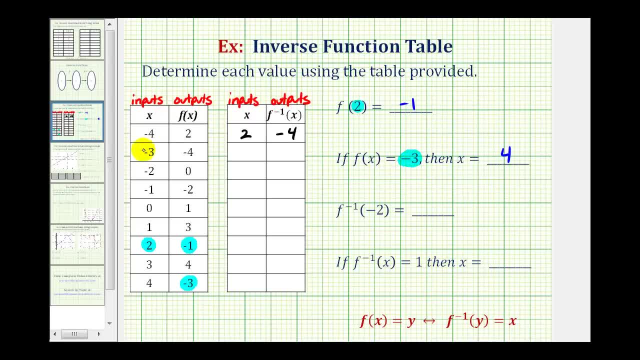 So we can see how these two functions undo each other. If the input is negative 3 here and the output is negative 4, then the input for the inverse function will be negative 4 and the output will be negative 3.. So we're inner changing the inputs and outputs. 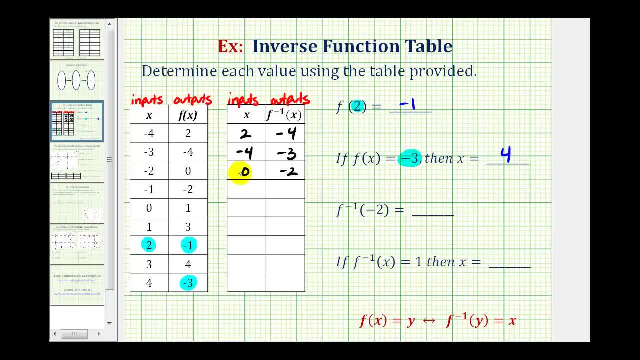 So this is negative two. zero, this is zero. negative two. If this is negative one, negative two, this is negative two. negative one. This is zero. one. this is one. zero. This is one. three, this is three, one. 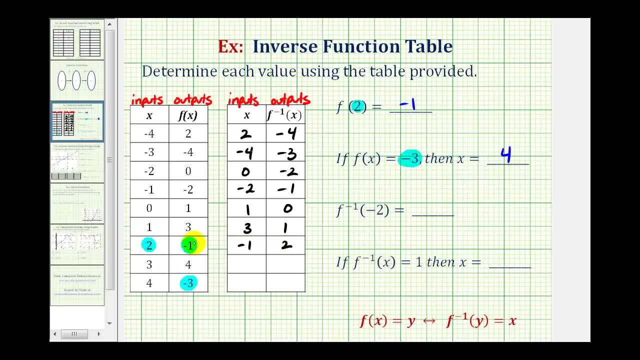 This is two: negative one. this is negative one, two, Three, four, four. three Four, negative three and negative three, four. So this table here should help us, on these last two questions, to evaluate f inverse of negative two.